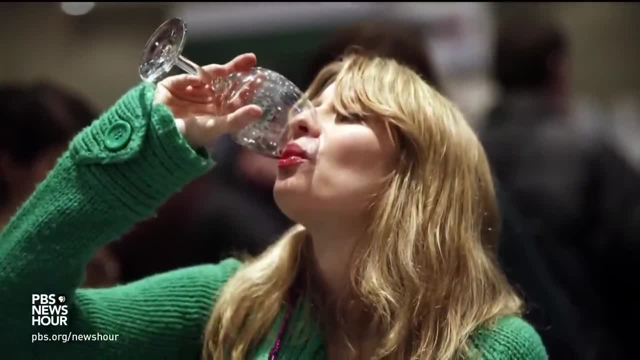 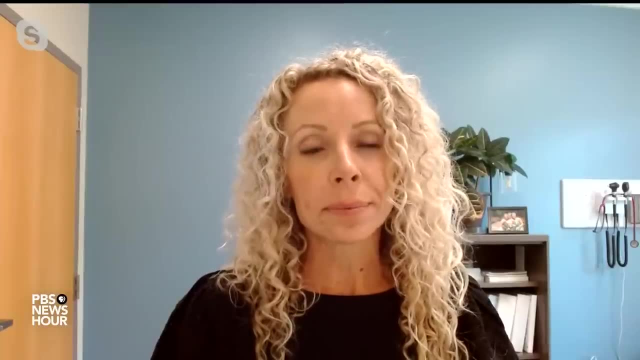 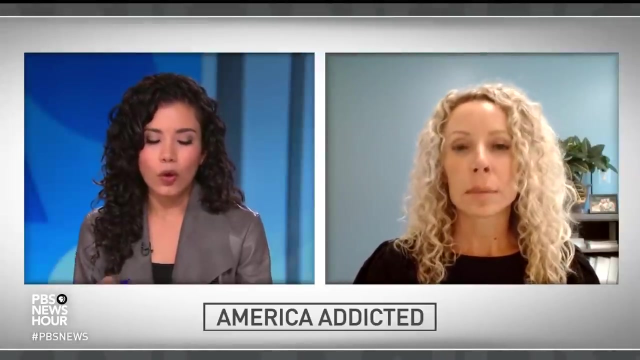 more and more alcohol use. Women are experiencing more stress, I think, in stress-related drinking as a result, And then I think the effects of social media has had its effect on women increasing drinking as well. LAURA BARRON- And the study specifically highlights the rise among women 65 and older. 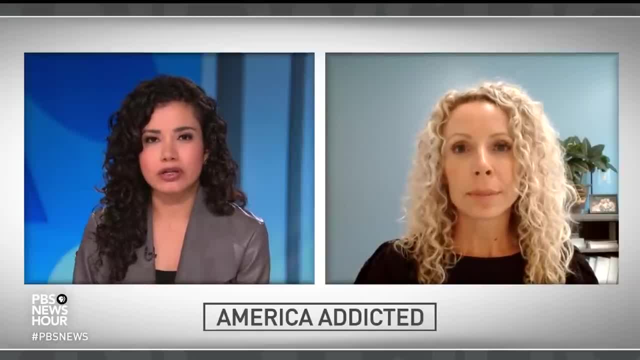 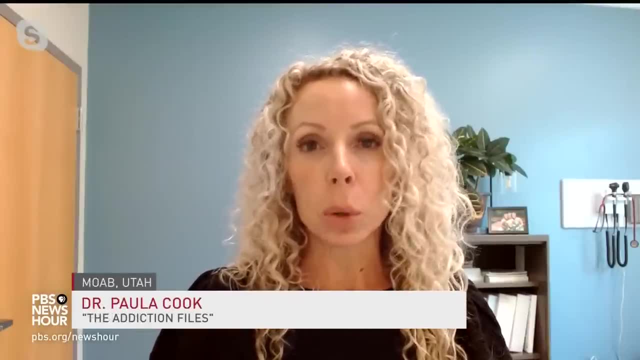 What could be causing that rise within that specific population? DR PAULA COOK, American Medical Association. Well, we're seeing increased substance use and alcohol use in the baby boomers in general. As they age, they're using more And this. 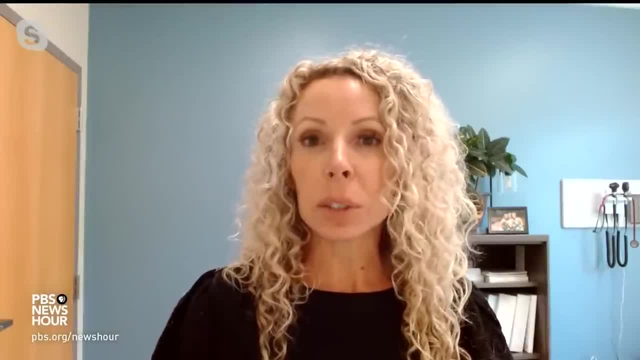 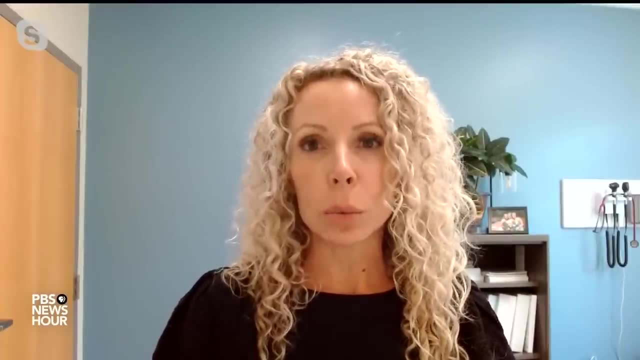 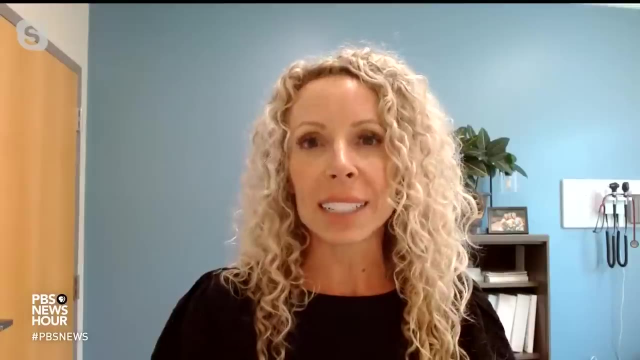 group of women particularly, are subjected to the same effects that we were just talking about: the marketing effects, the stress effects, And as they leave the work force, there's interesting effects of women in terms of increased rates of anxiety, depression, et cetera, and more likely to reach to alcohol to kind of mitigate some of the effects of 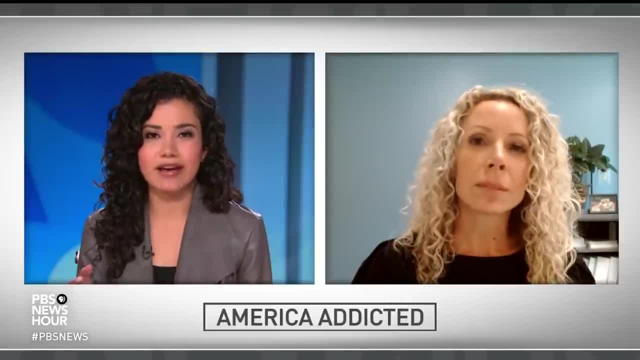 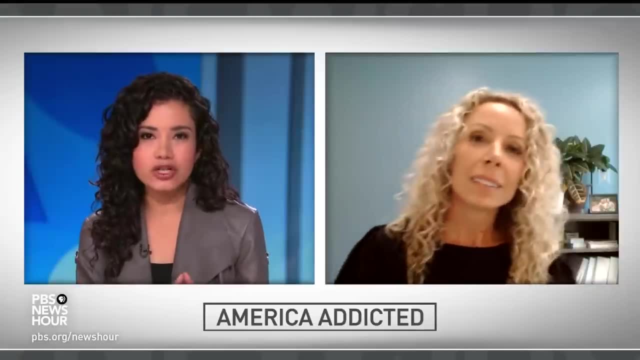 that, LAURA BARRON- There's been some studies in the past that have told the public that one glass of red wine a night is OK. But how much drinking is OK Is too much drinking? Because some of the dietary guidelines say that one glass a night. 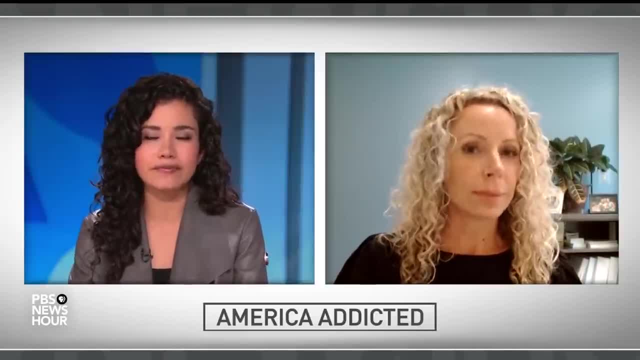 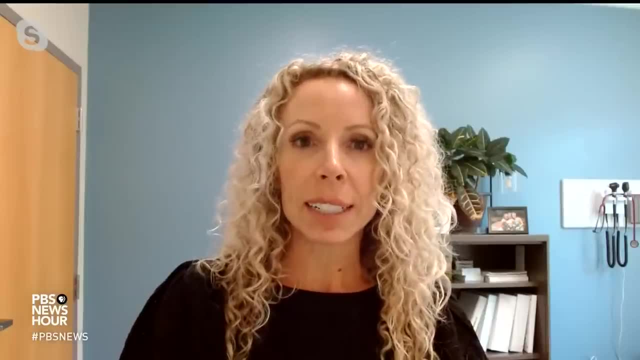 for a woman is OK, two for a man is OK. What do you say, DR PAULA COOK, American Medical Association? Well, this has been very confusing, But lately the American Heart Association, the American Cancer Society, have come out with really clear. 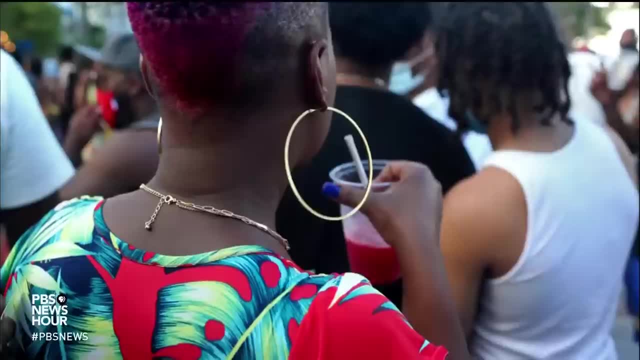 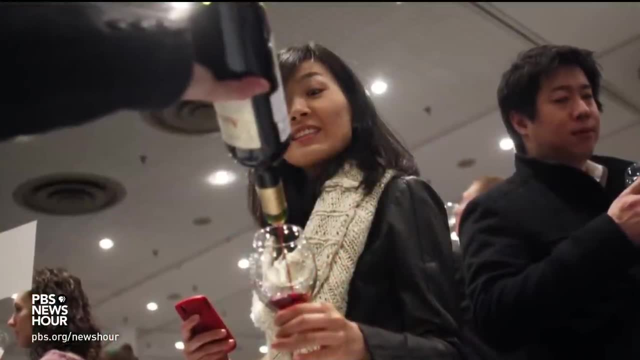 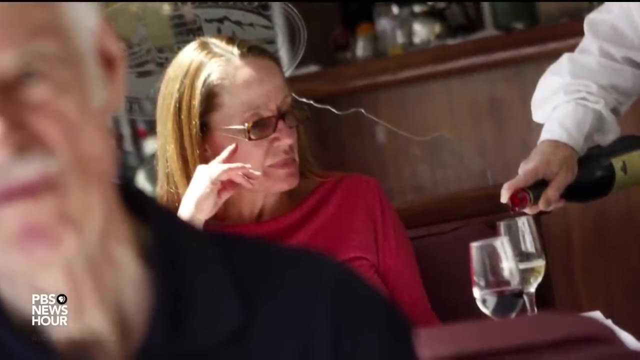 guidelines saying that really no alcohol is safe. So before, when we used to say maybe a glass of wine at night was helpful for your health and your heart, especially now, alcohol has more risk than benefit, And so, even though moderate drinking may be OK for some people, one drink for women. 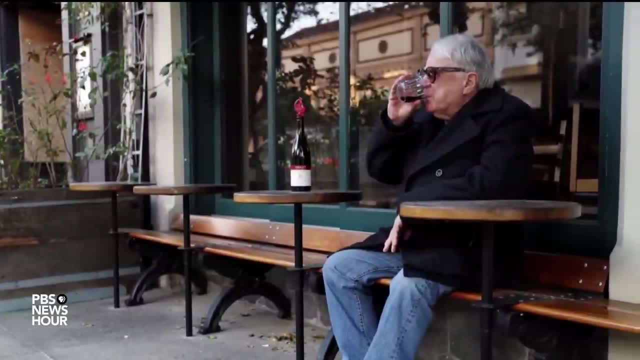 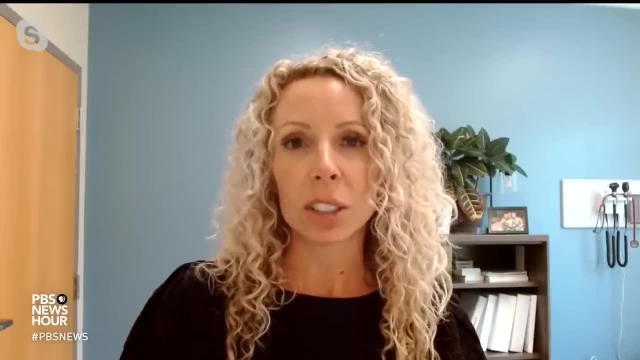 or less, two drinks or less for men. there are many people in the population who shouldn't have alcohol at all And the health benefits of alcohol have really been negated in the research. LAURA BARRON- What happens, physiologically speaking, when women consume alcohol? 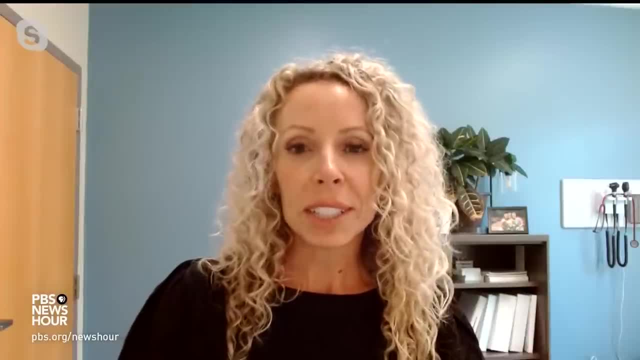 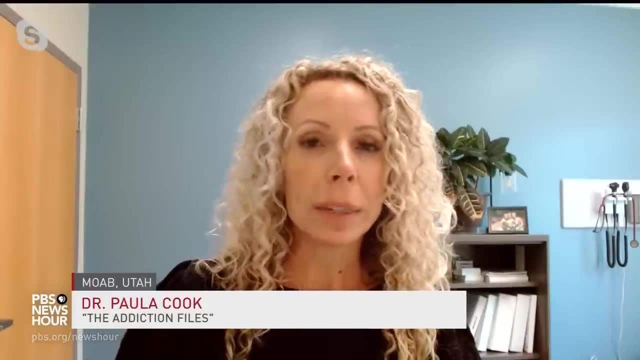 versus when men consume it. DR PAULA COOK, American Medical Association. Well, there are several differences. I mean women, both chemically and physiologically in their bodies, handle alcohol differently. So women have a higher body fat percentage than men, who have more water content. So alcohol